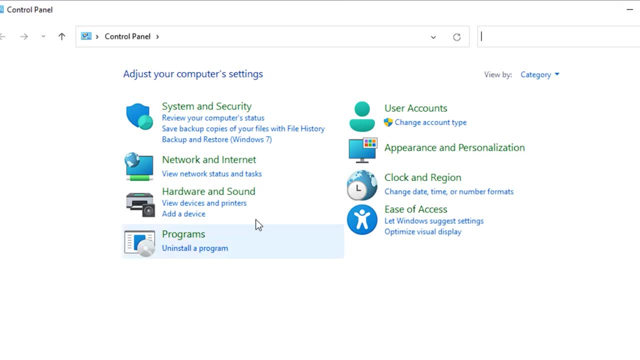 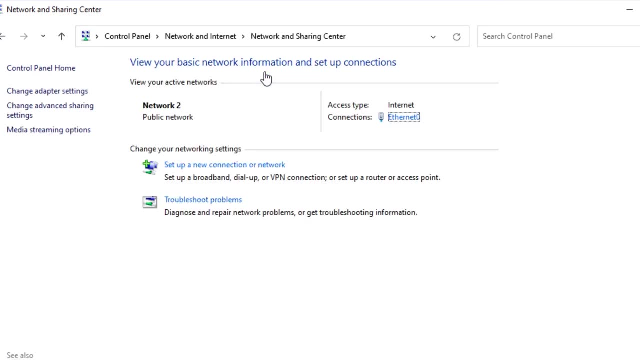 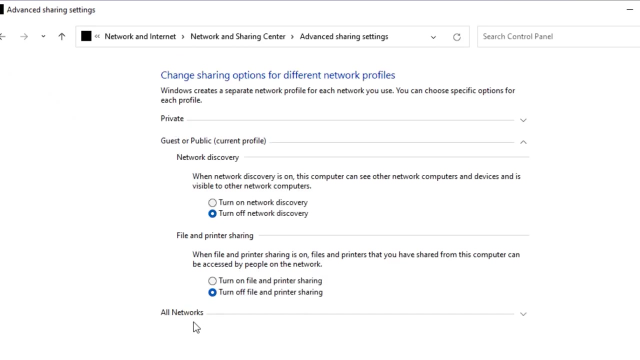 control panel and you will find network and internet. click on that. then find network and sharing center. click on that. you will find change advanced sharing settings. click on that now you'll find private, guest or public and all networks tabs under the private, select. turn on network discovery. 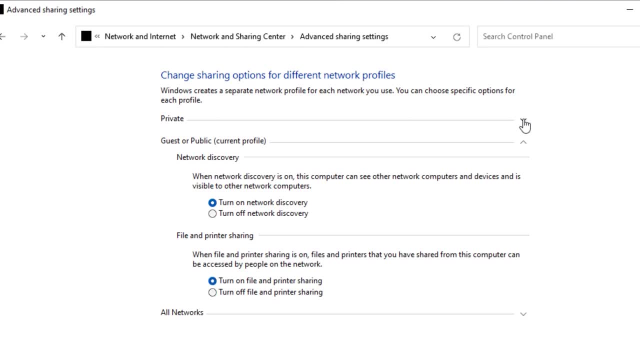 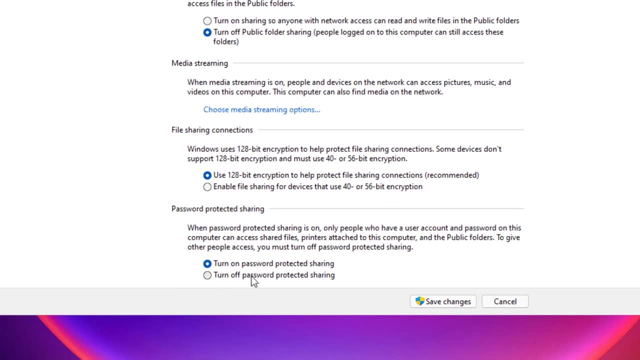 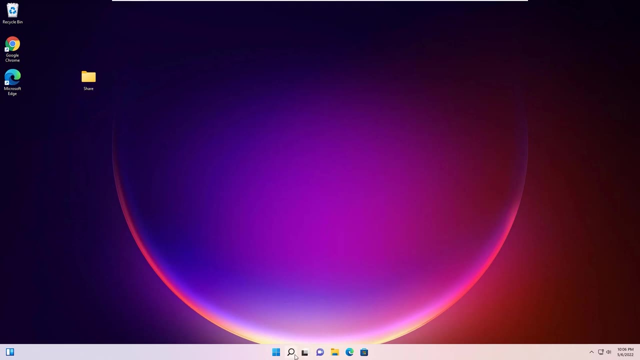 and turn on file and printer sharing. now expand the private here also turn on everything. then finally expand the all networks. here select turn off password protected sharing. then save changes. now close the window. as a second step, again open the windows search bar and search for services. we'll find. 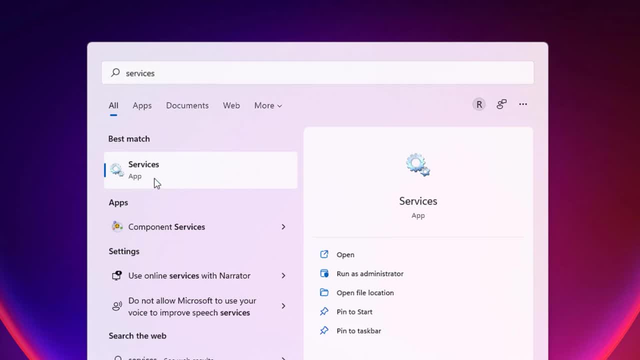 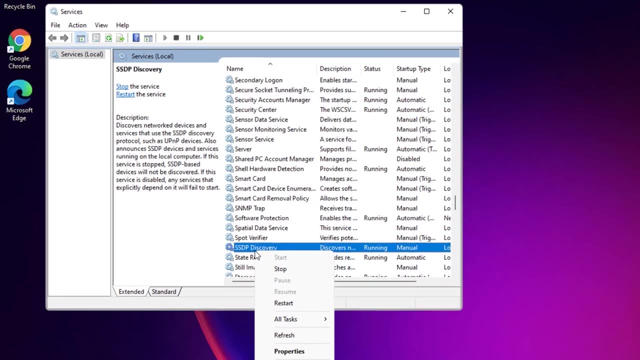 services app under the best match results. click on that. now you need to find ssdp discovery. you will find ssdp discovery right. click on that and select properties. now in the startup type. by default it's set to manual. change it to manual and then click on the all network tab and then you will find all networks. 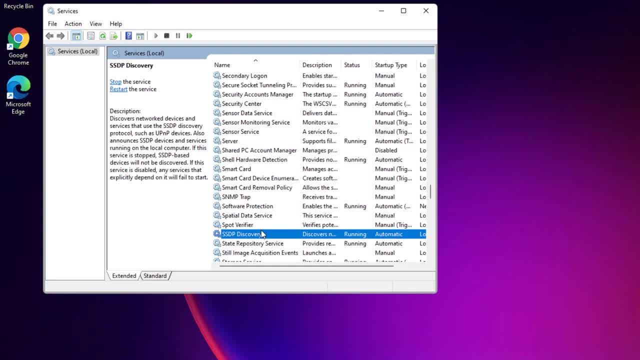 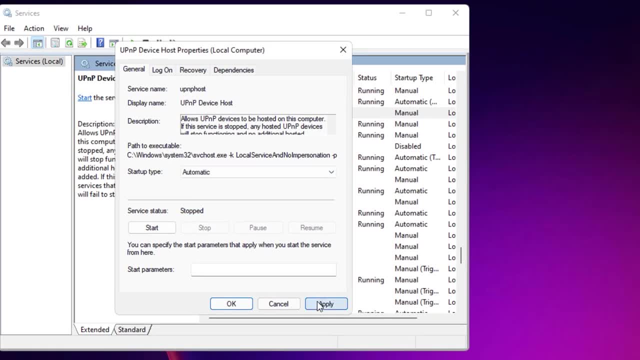 until now it's there. right click on it is set to automatic. then press apply, then say ok. again search for upnp device host. right click on that and select properties. change the startup type to automatic and apply. say ok. then find functions: discovery provider host. right click on that. 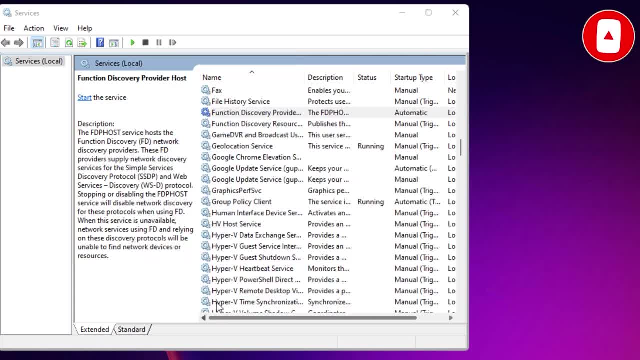 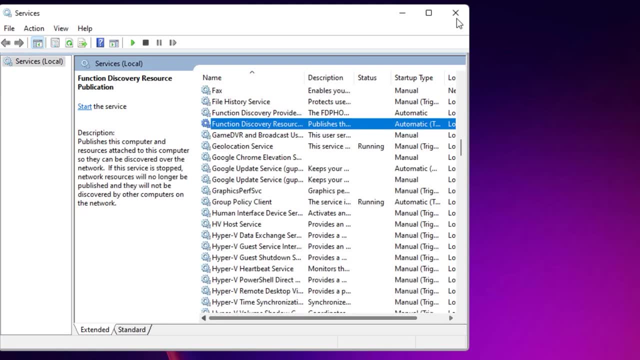 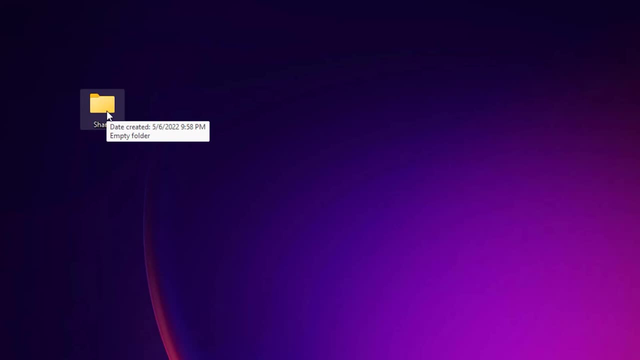 and select properties, change it to automatic and apply. ok, like that for function discovery resources: right click properties: automatic apply ok. so once you're done, close the window. finally, we share the folder by performing the final steps. that is, right click on the folder which you want to share and select properties. then you will find sharing tab. click on that now in the advanced. 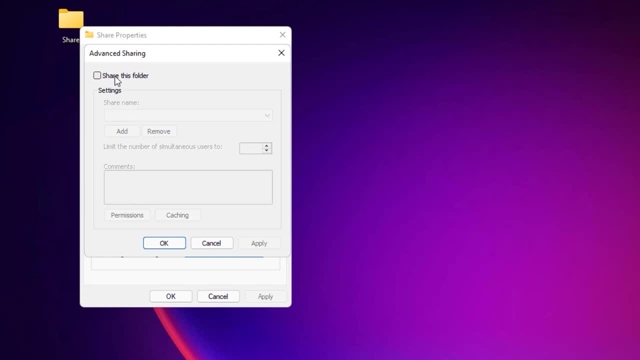 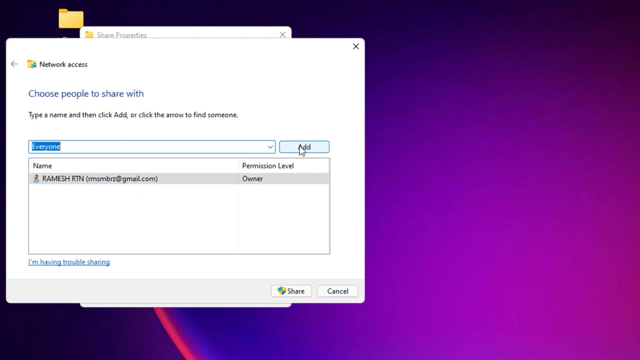 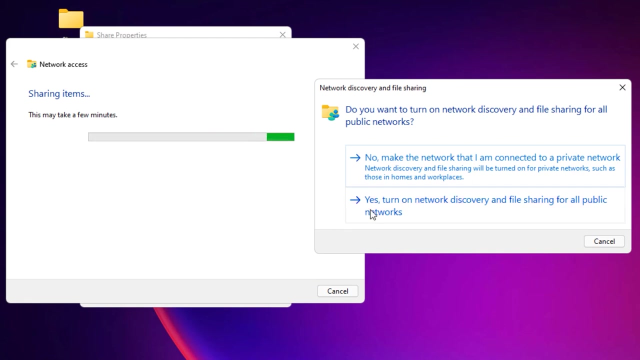 sharing. click on advanced sharing button. then select share this folder. now select permissions. select the all under allow button, then apply. now say ok again. then finally you will find share button. click on that. select the drop down to everyone and add now in the permission level. select it and give read and write. then share. now select yes. now we have successfully converted the.